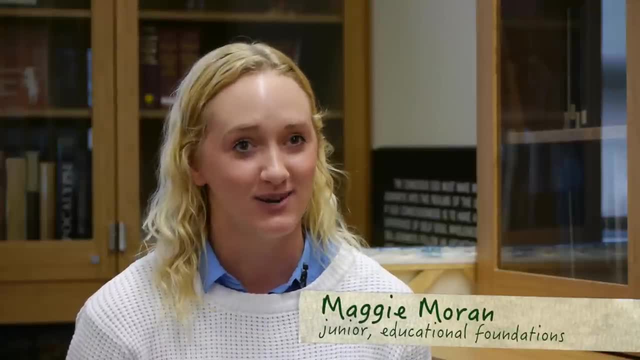 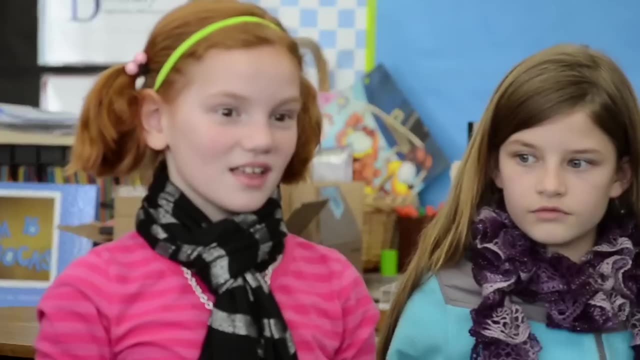 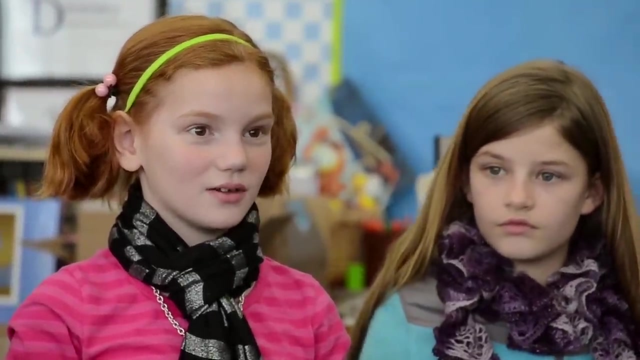 crickets in the background And much to my surprise and joy, it was not. They ran with it. If you buy something and that makes you happy, that happiness won't last forever. It will make you happy at first, but as your life goes on it will start to come like just as regular things. 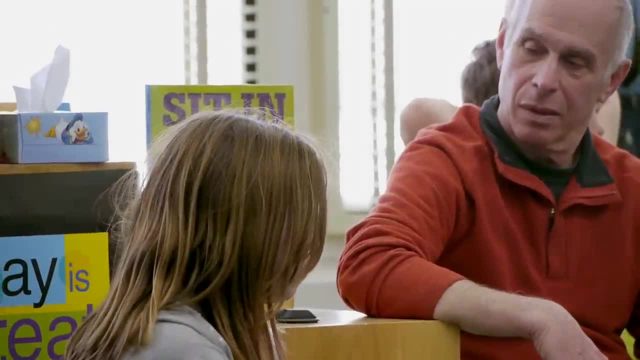 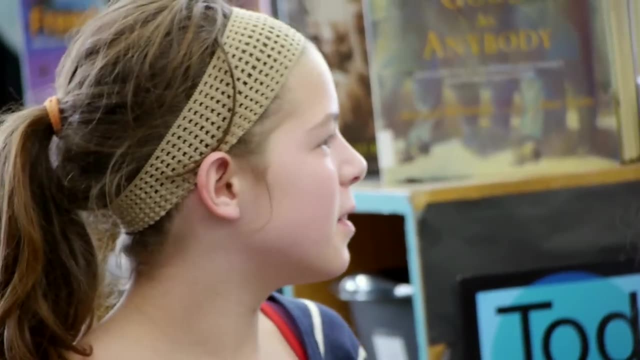 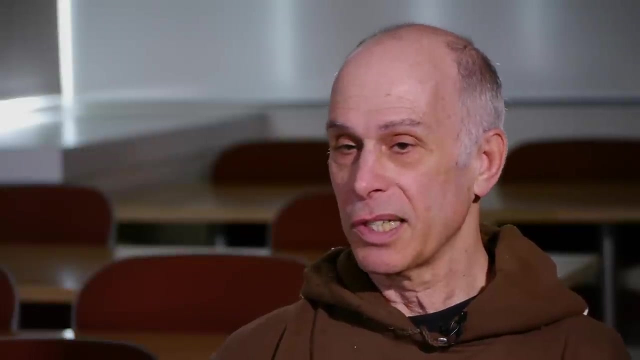 We promote critical thinking and putting a context to facts so that kids, when they're doing, when they're trying to make sense of something they read or something they research, that they're going into more depth rather than simply regurgitating facts for assessment tests, for example. 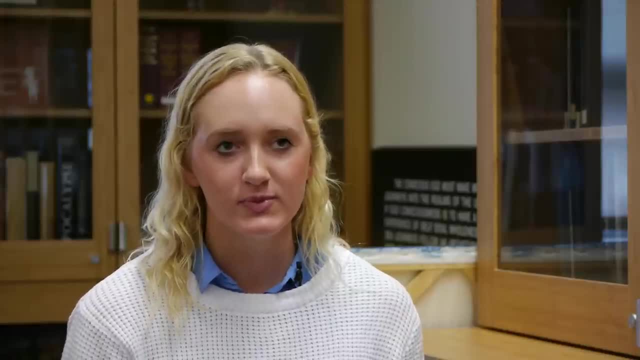 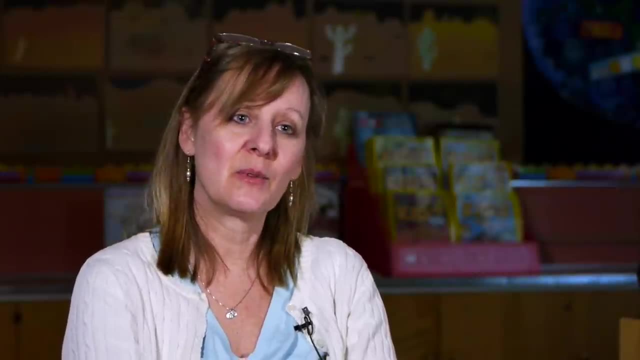 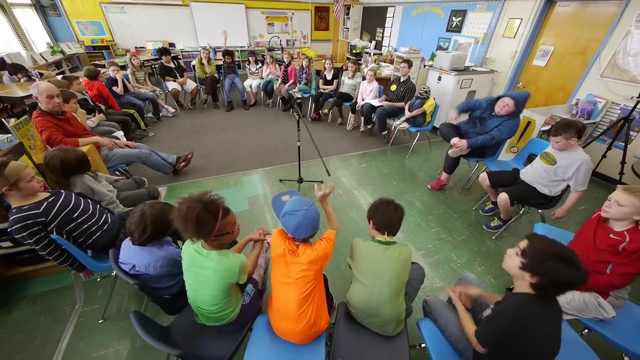 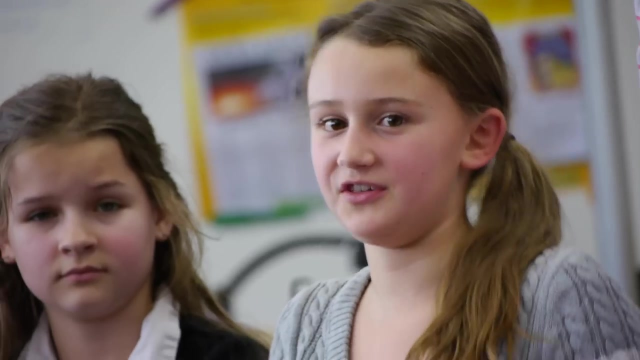 Encouraging all of those thinking processes helps young kids across the board. Mostly what I got out of it was seeing the kids have this opportunity and having the students recognize this ability in themselves, Being, you know, in a position to be in college and tackling tough issues, and you know. 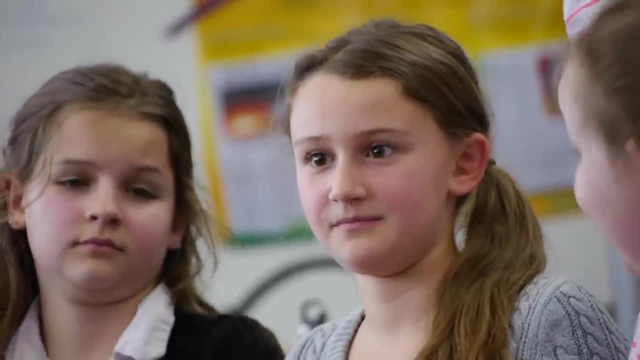 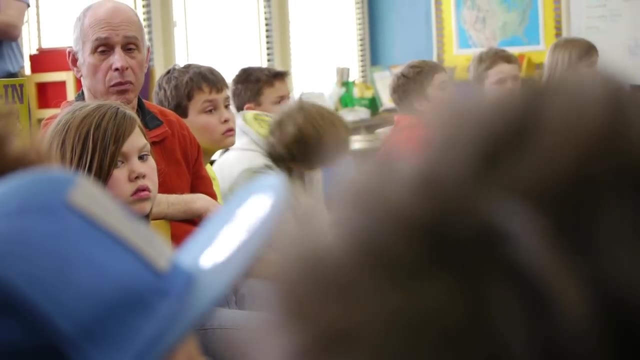 that's so invaluable. You can't put a price tag on what that does to a child's self-confidence. We study the art of teaching. How do you make sense of an opinion, back it up with personal experience, which is very hard for kids to do sometimes. 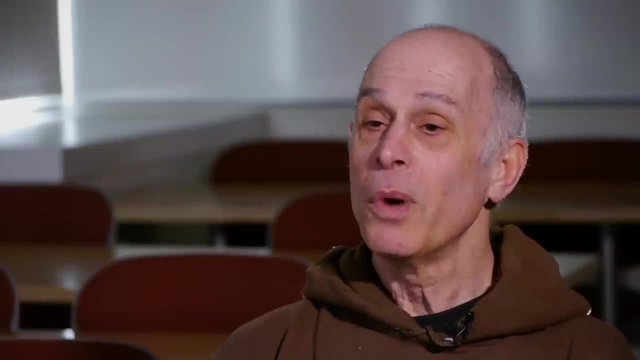 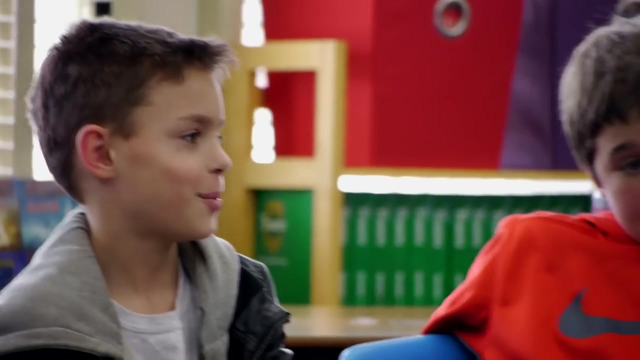 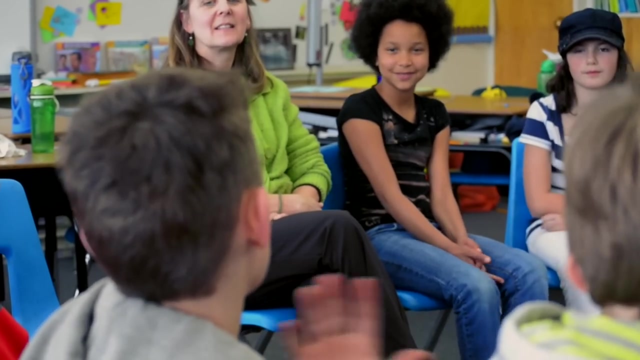 and then revise your position based on new evidence that you've received from a peer in a circle discussion. This changed my perspective because of you. How do you explain like: can you be happy? Like money-free, happy, Yeah, And then just happy about it? 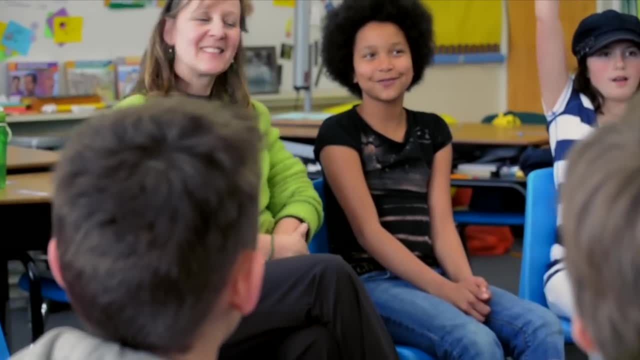 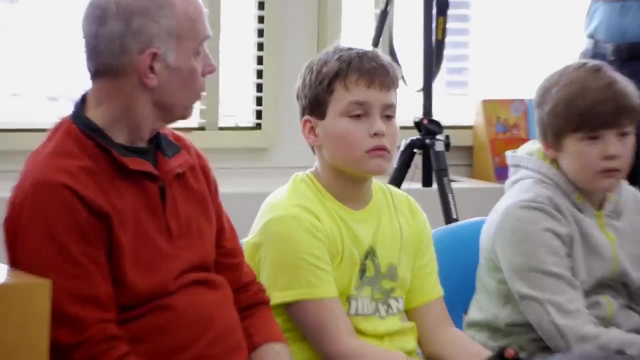 Yeah, Like waking up in the morning and just happy that you're alive. The students themselves see each other differently. That's one of the coolest pieces is like maybe kids who struggle with some of that core subject, With reading or with math. 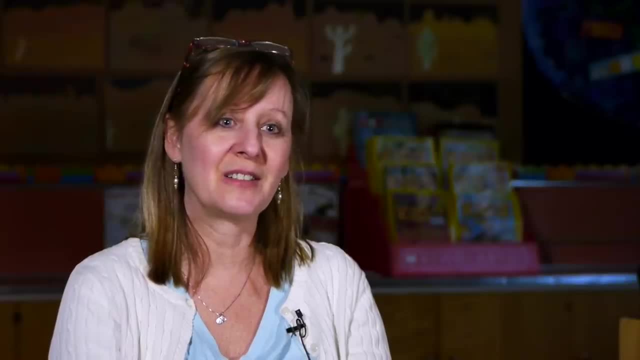 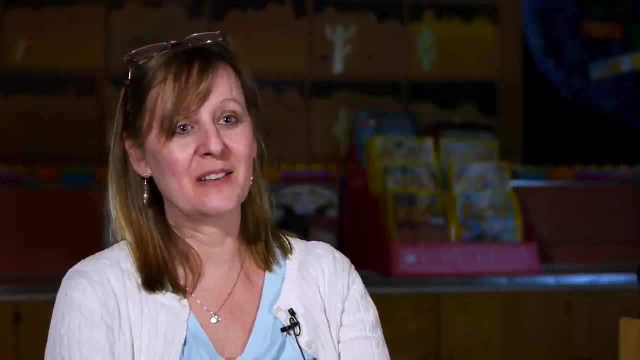 And they come down here in this circle and they have these profound life things, you know, like wow, kind of comments And it's so good for them and for their peers to see them in that different light. Okay, go ahead.